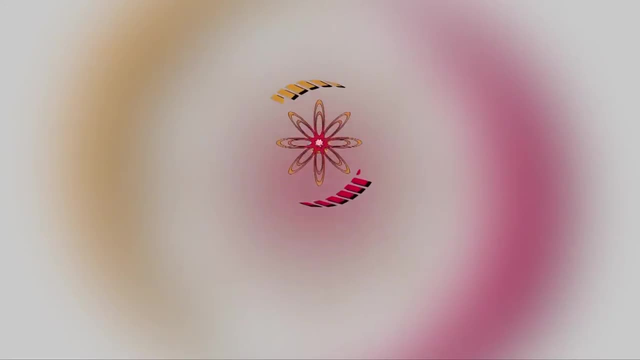 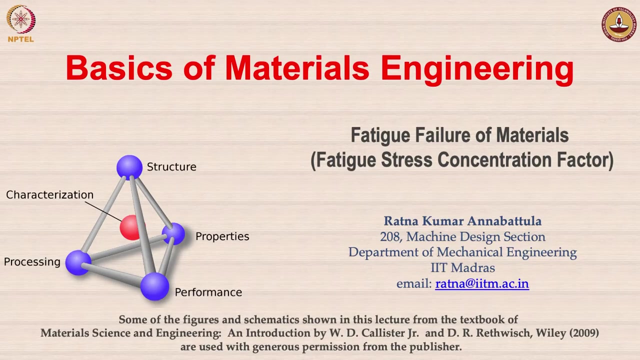 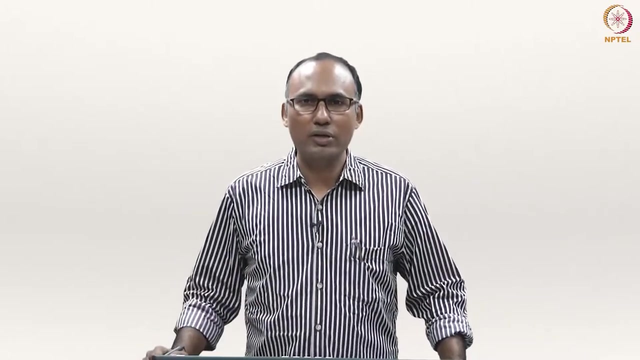 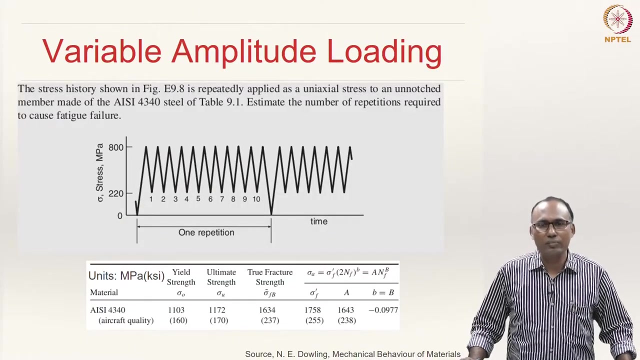 So in the last class we have looked at Variable Amplitude Loading and Multi-Axial Fatigue Loading and so far the material that we have covered, as far as fatigue failure of materials is concerned, is under the assumption that there are no notches or stress rises. We have not. 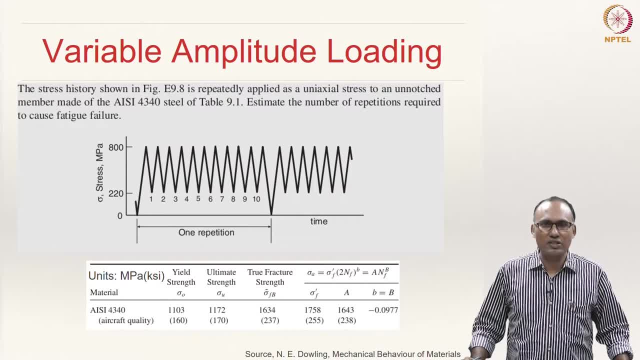 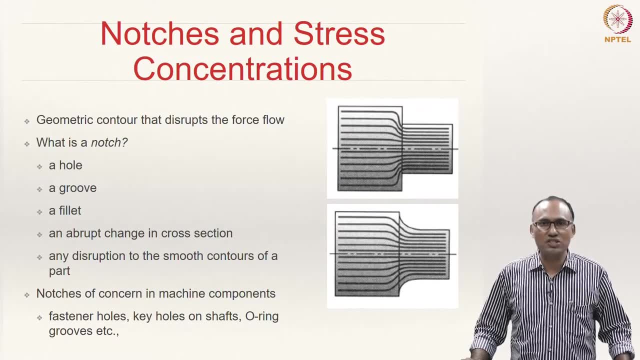 focused on the fact that there may be some stress rises within the component, And now, today, we will look at the situation when you have notches and stress concentration zones within the material, and how do we go about dealing with them. right, So what is? 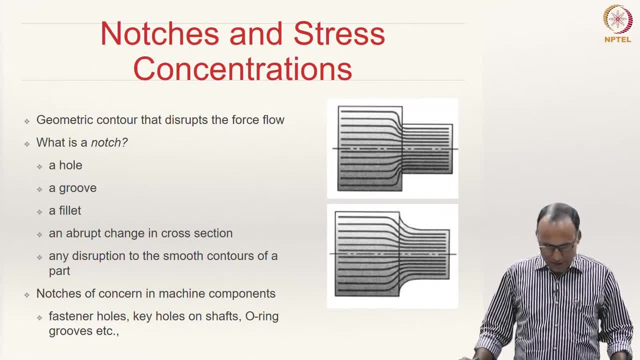 a notch, as we have already discussed during static failure theories, where, when we are, we have defined something called theoretical stress concentration factor. there we have discussed, we have seen this figure already. So a notch is something, or a stress concentration zone is something, that has a, which is actually a geometric contour that disrupts the force. 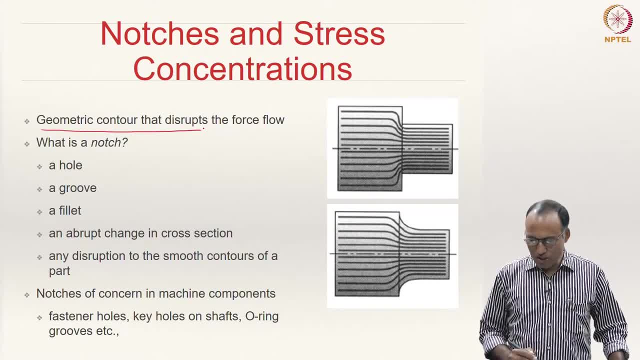 flow. So you can, as we have already mentioned in previous classes, that you can- take an analogy with the stream lines when we are doing the fluid mechanics course, you probably heard of this- streamlines. So when you have a change of geometry, the streamlines get closer and similarly, here you can represent them with 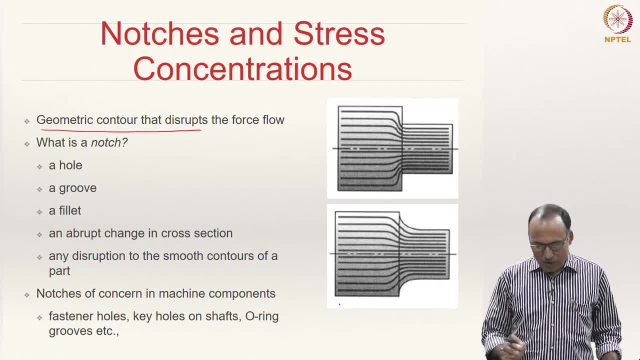 the. you can do a similar analogy between streamlines on the force flow lines, right. So, as you can see the figure, this figure actually shows a sharp change in geometry. as a result, the distance between the force flow lines is much less compared to when you. 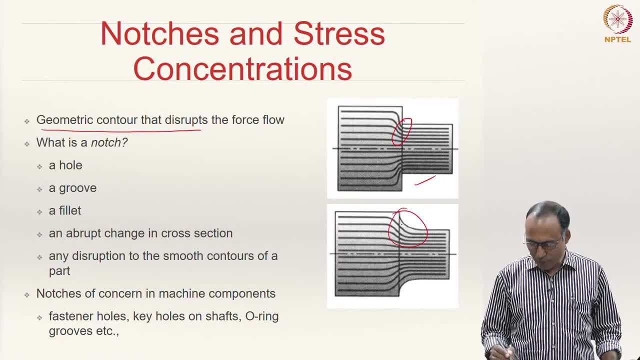 have a gradual change in geometry where in the distance between the streamlines is much less disrupted compared to here right, So which otherwise means that this represents a very high stress concentration zone compared to this situation. So what are the different kinds of? 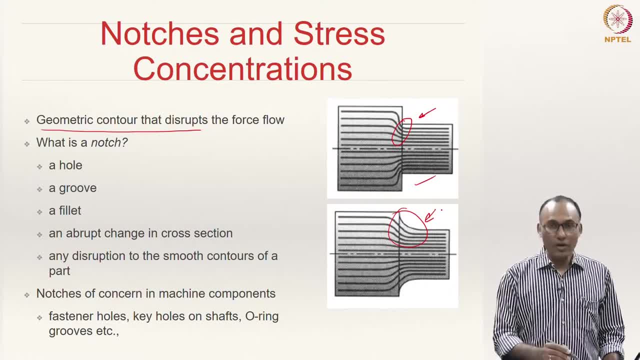 So notches that we will come across. in machine components, for instance, you may have several holes. a groove, a fillet, an abrupt change in cross section, a keyhole and so on are, in general, any disruption to smooth contours of a path can be considered as a notch or a stress riser. 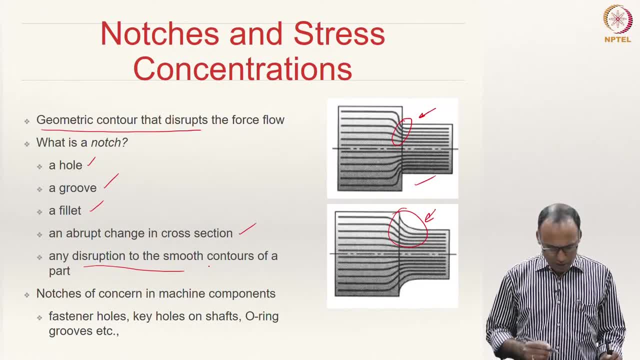 And in machine components the typical features that can be considered as notches and should be given So we can see that a tight notches is a notch, is called a notch, or a stress riser can be considered as a notch, So it may be a notch or a fillet, or we can see that it is a notch, so this is called a. 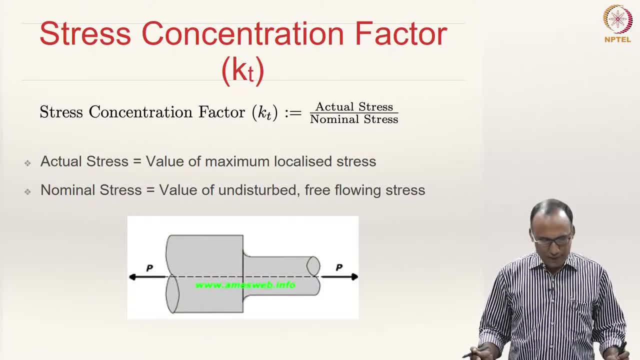 notch or a stress riser, So it has to be taken care of to. So you can consider a for field load, as in this picture. so this is the for field load divided by this cross sectional stress. So the stress is a for field load. 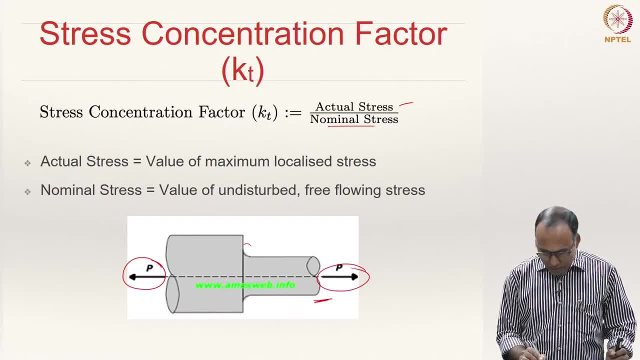 So what we have decided, So what we will do, So that is your nominal stress. and what is the actual stress? because of the stress riser that is present here, the stress at this position, divided by the far filled stress, is your stress. 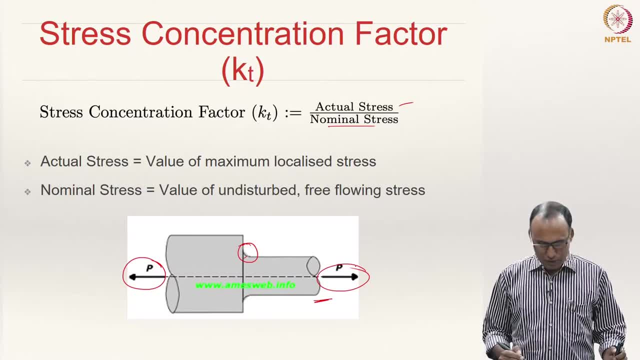 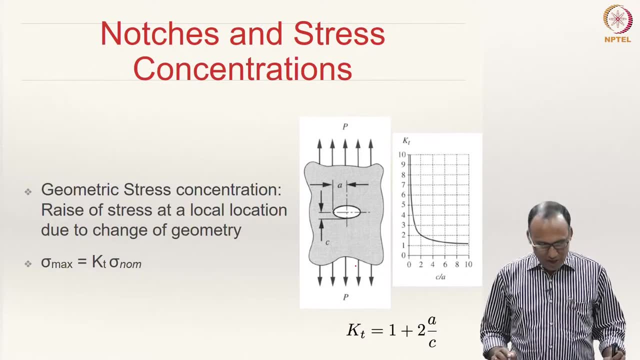 concentration factor. So that is what is called theoretical stress concentration factor or geometric stress concentration factor, and we have seen, for different kinds of geometry, of the whole shape and size, we have the formula for finding out the theoretical stress concentration factor. For instance, here you have an elliptic hole whose major axis, semi-major axis, is A, and 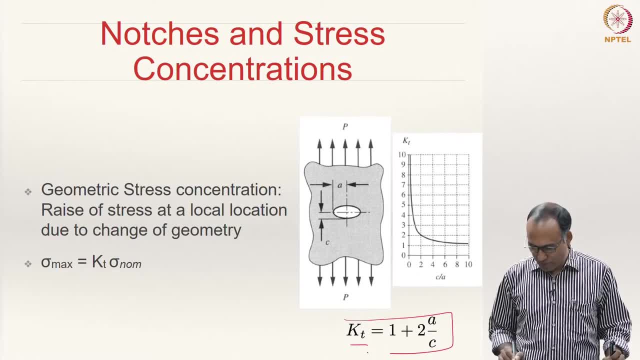 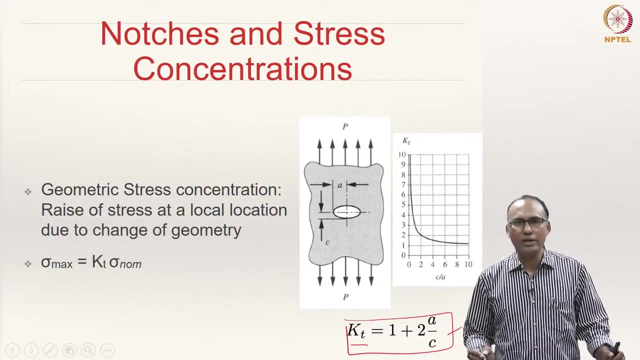 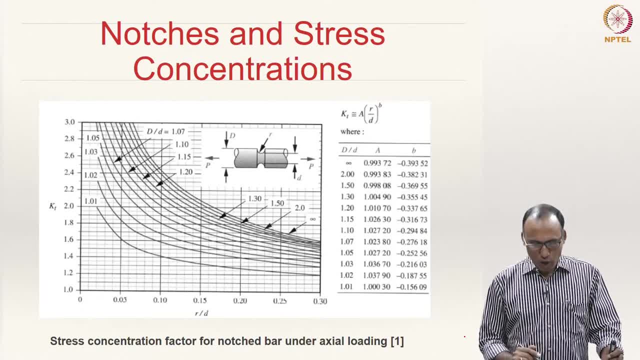 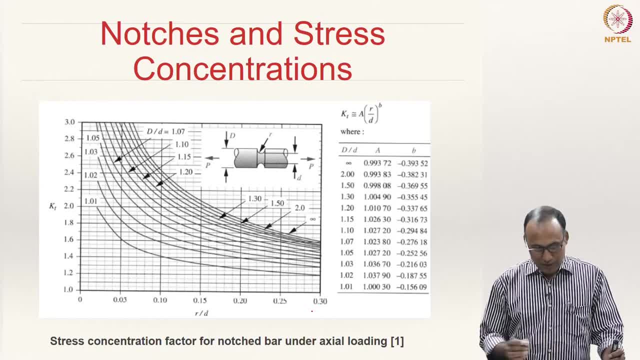 factors, that people have actually derived these empirical formula or have done several experiments and came up with these charts. All that we need to do is now you look at the appropriate chart, based on the type of the notch and the type of loading, and then calculate and then identify the stress concentration factor and then use that to estimate the stresses. 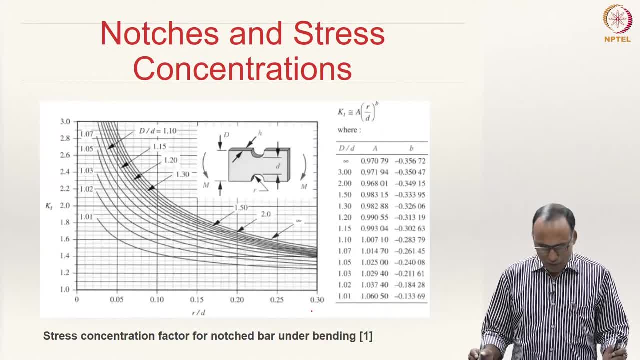 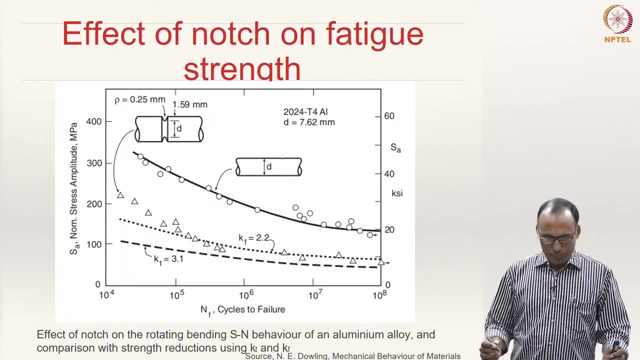 in a particular region in your machine component, So this is for bending, and where your cross section is a rectangular cross section, and so on. So here this graph nicely summarizes the effect of stress concentration on the fatigue strength. So here the solid black line represents a fit to the fatigue strength life diagram. 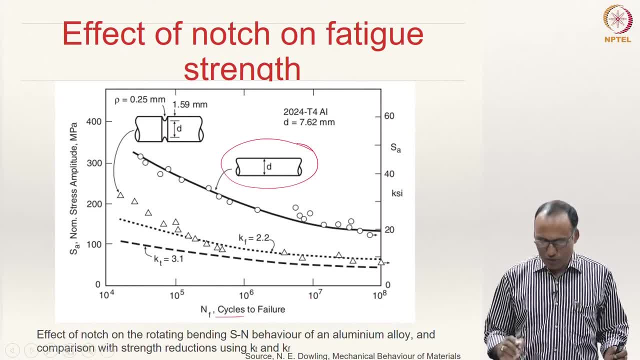 for a unnotched aluminum specimen of 27.62 mm diameter. So, as we know that you will not have a perfect line matching all these things, because of the variabilities in the crack structure in the material, We have seen that there is going to be always fatigue any. 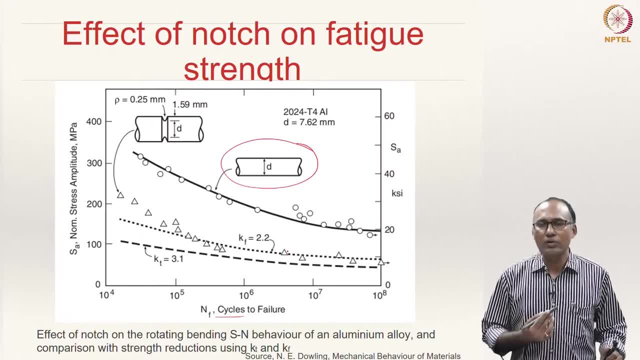 experiment will have some error bar and fatigue failure also will have usually a larger error bars. So this is the situation when there are no stress concentrations and now you have a same shaft with a notch, a groove in between. the radius of that groove is 0.25 mm, and then 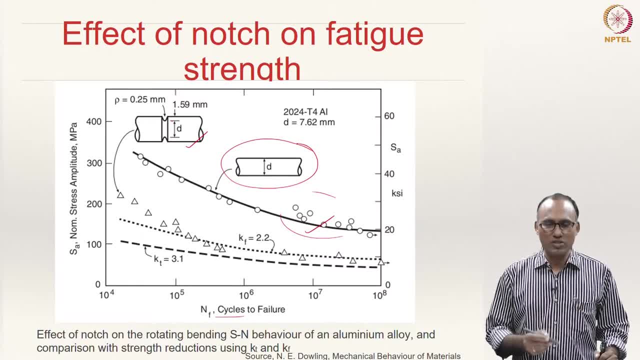 you do the again, the fatigue loading on this specimen, and then try to develop SN curve, You can clearly see that suddenly there is a sudden reduction in the strength of the material. So on the y axis we have a stress amplitude and x axis you have a number of cycles to 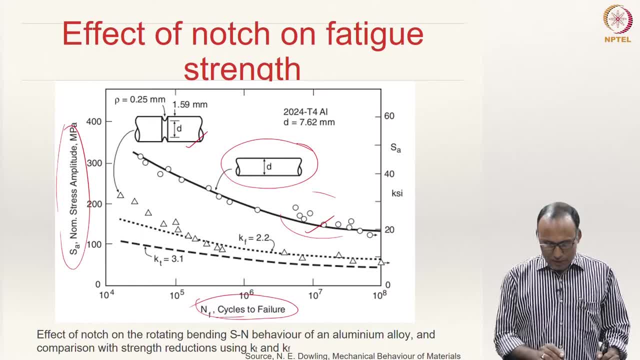 failure and you can see that the fatigue strength of this material is much less than the one that which does not have a crack. However, if you would calculate the theoretical stress concentration factor of this material and if you simply multiply the theoretical stress concentration factor with the stress calculated from the far field stress that is available, 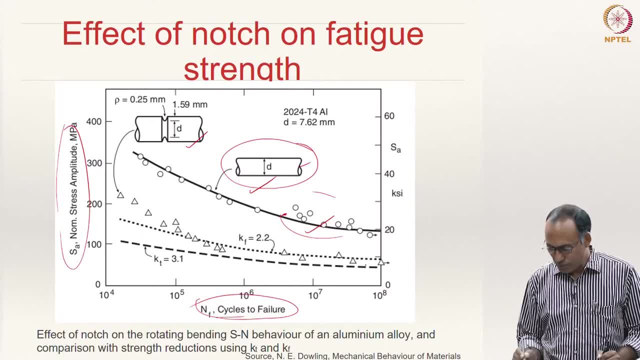 So you can see that the fatigue stress concentration factor is much less than the one that is applied on this. the curve that you will get from this solid curve will be this dash line, where k t equal to 3.1 for this particular configuration. However, when we do the experiments, it turns: 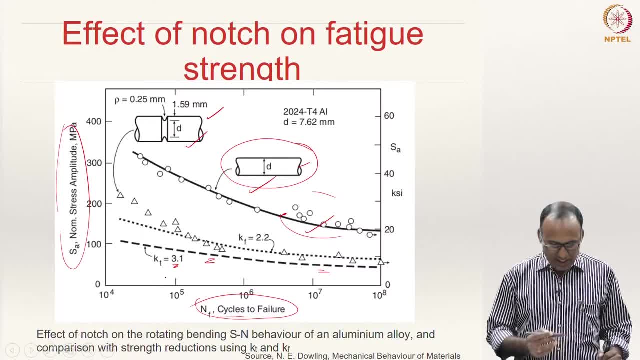 out that the fatigue, stress concentration, fatigue strength of the material is actually little higher, little bit higher than what you would have calculated by using your theoretical stress concentration factor. And if you would calculate the stress concentration factor- fatigue stress concentration factor- directly from the geometry, you will get 3.1.. However, 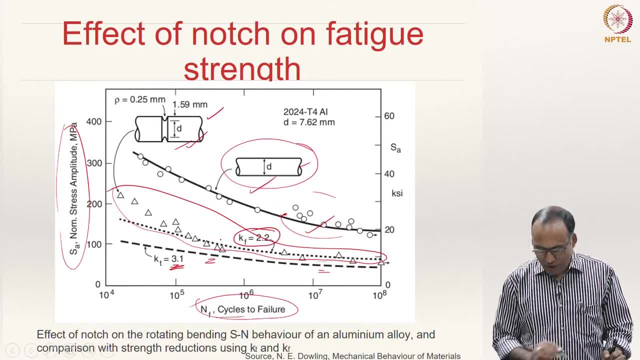 after measuring. if you fit this line, then you would figure, find out that the fatigue stress concentration factor represented by k f is actually 2.2, which is less than k t. that is how you one would observe. right. So now, why is that? the fatigue stress concentration? 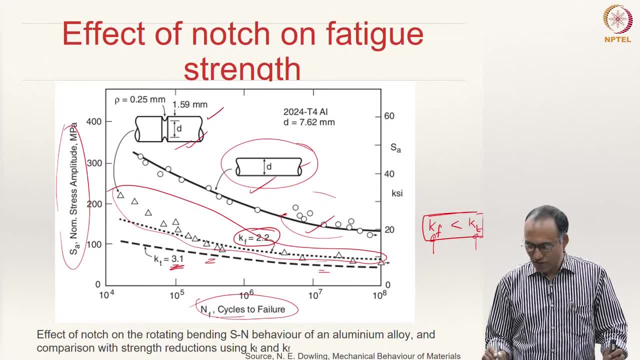 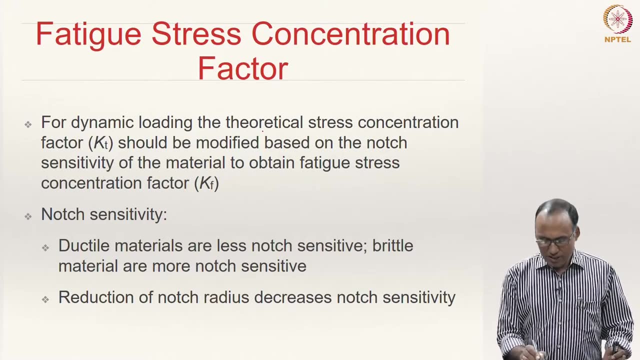 factor is very different from theoretical stress concentration factor and further question is that: why is that fatigue stress concentration factor is actually lower than the theoretical stress concentration factor? So for dynamic loading the theoretical stress concentration factor k, t should be modified based on the notch sensitivity of the material. 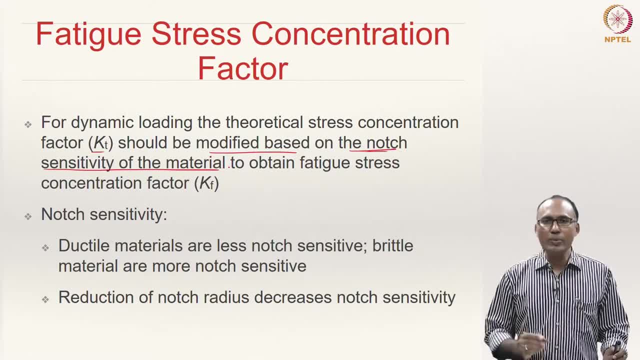 there is something called notch sensitivity, So that needs to be accounted for when we are talking about stress concentration factor. So when we are talking about stress concentration factor and hence you cannot use theoretical stress concentration factor, you have to use a modified theoretical stress concentration factor for fatigue loading, and that is called. 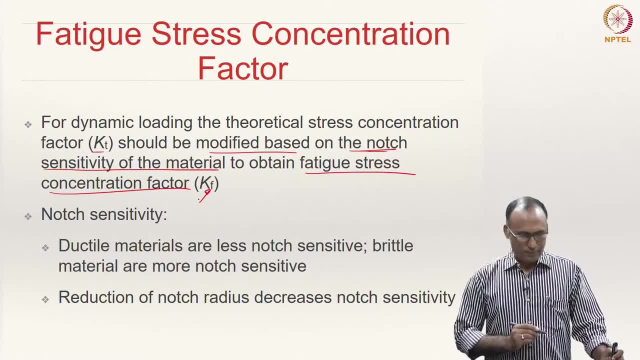 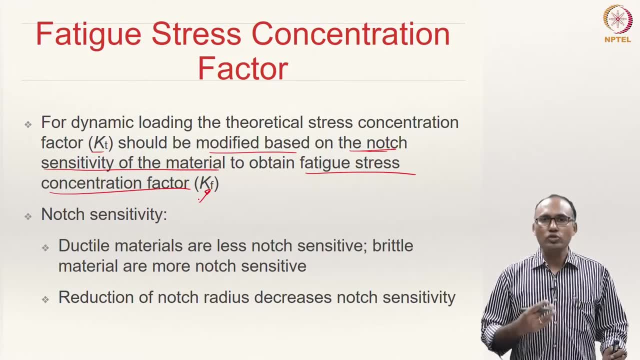 fatigue stress concentration factor represented by k f. So notch sensitivity is the basically the sensitivity of the material to the geometry of the notch, particularly when you have fatigue loading, and this sensitivity is actually material dependent. IntegralConcentrationFactorKft crux-achevolumeq買付做 Salt shifted into 0 for Federationof. 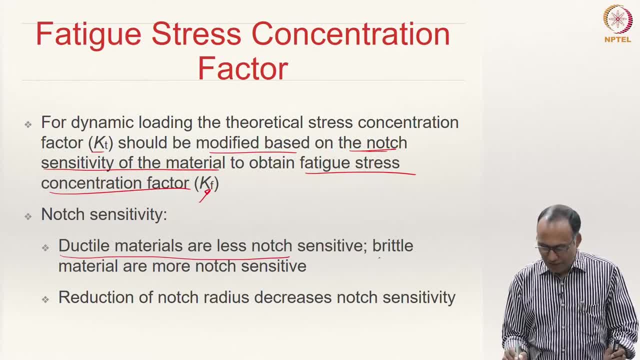 Free St. Assimilationcheckersfautohjahrischaperco- loginetextjpg. е- m, defectiv, Нет. Significance gibt Es und Nicht sein. mit der Lehet ABvN. an solidarity basis ist 1 and telling the less for ductile materials and very high for brittle materials. So brittle materials are. 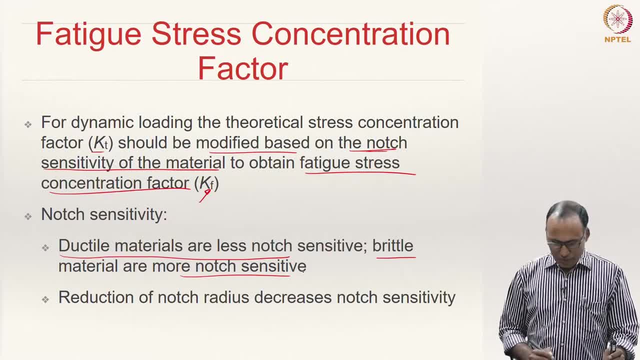 more notch sensitive compared to ductile materials and, as you, when you reduce the notch radius of the notch, then the notch sensitivity decreases, because when you reduce the notch radius, you will increase the plastic deformation ahead of the crack tip and that will lead to making the material get into the ductile regime, because you are introducing plastic deformation and 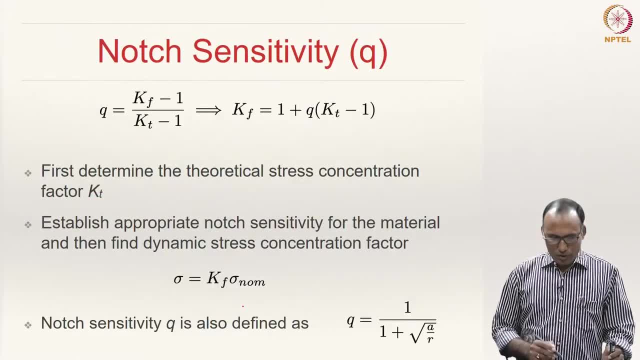 hence they become less notch sensitive. So this is the correlation between the notch sensitivity, Q, fatigue stress concentration factor and theoretical stress concentration factor. So by knowing the notch sensitivity and theoretical stress concentration factor one can obtain fatigue stress concentration factor. So the work flow when we are doing. 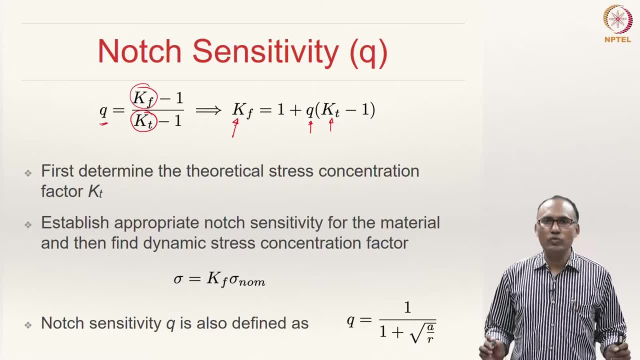 the design based on fatigue, So components which have stress risers or notches. all first thing that we need to do is first determine the theoretical stress concentration factor from the charts that are available or from the empirical formula, and then you establish the notch sensitivity. 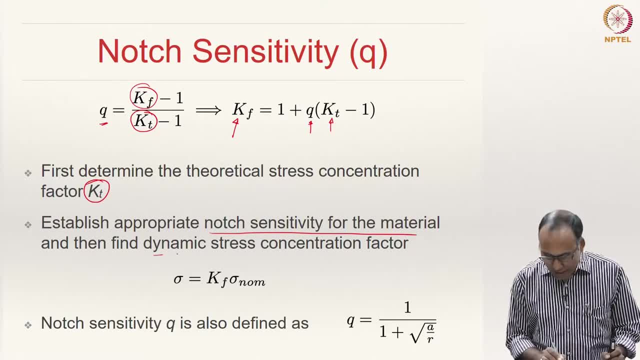 of the material and then find dynamic stress concentration factor or fatigue stress concentration factor. How: once you find K T and then you find Q and plug that in this equation, then you get the K F, And once you have K F you multiply that with the nominal stress to. 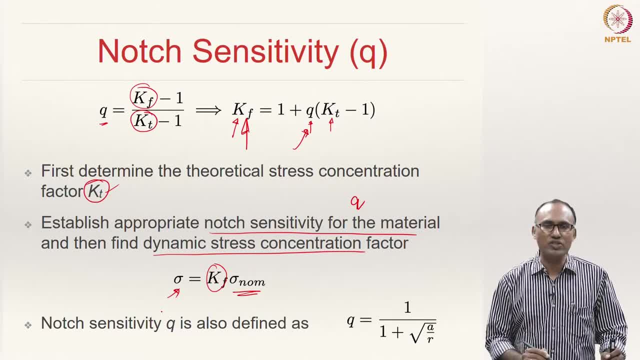 get the actual stress experiencing by the component at the position where you are actually calculating the stress concentration factor. So the notch sensitivity Q can also be defined in terms of the geometry and another parameter called a. please note that this a is not crack length. We have been using a for the weight, So you need to have stirring or camelivering. Now please note that you need to haveie trailing. So the way that you can terrible move this a nothing knowing the torque of it or not, you will find that the H minus H by感謝ize, maybe minus T. Also, you need to have fill degrees called, lol, so percents, time size being. 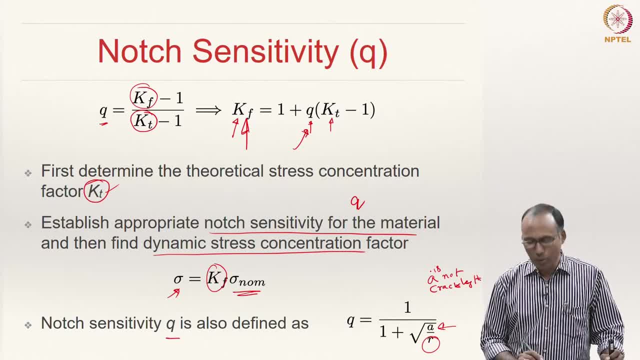 crack length when we are talking about fracture mechanics. but here this A is a constant that comes from material property or the ultimate strength of the material. So your notch sensitivity is a function of the geometry as well as the material property. and this constant A, or in. 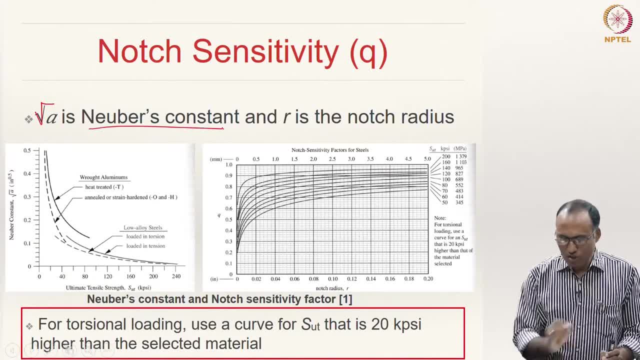 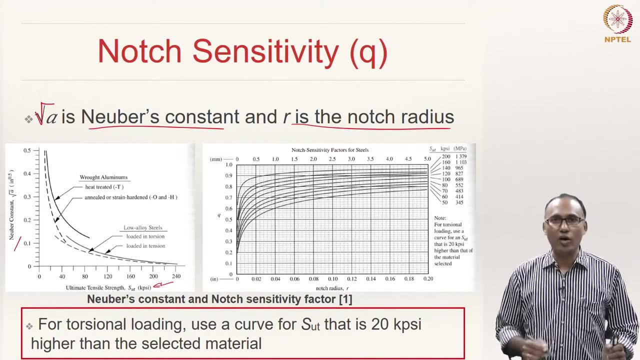 fact, square root, A is called Neuber's constant and R is the notch radius, and the Neuber's constant is dependent on ultimate strength of the material. For different materials, the Neuber's constant is different. right, You have graphs like that or tables from which you can directly calculate the Neuber's constant. We can 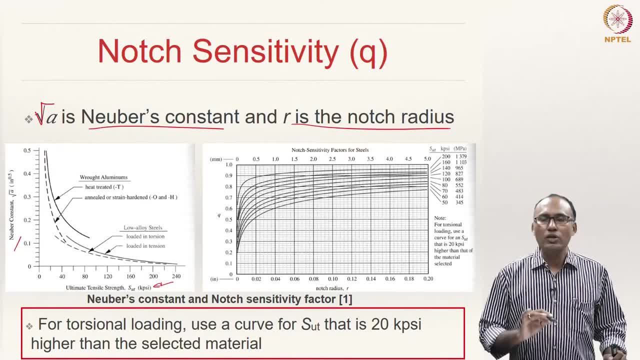 see that in a moment. and then, since we know that Q is a function of Neuber's constant, square root A And the notch radius now for different kinds of…. So Neuber's constant here depends on the ultimate strength of the material. So here, this graph here shows notch sensitivity. 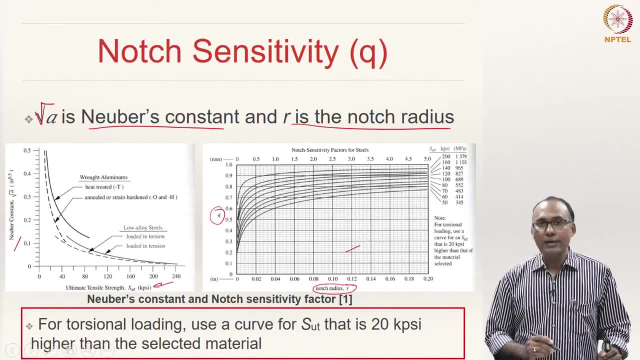 Q as a function of notch radius, and the effect of material property is plugged in here through different curves. here Each curve represents a particular ultimate tensile strength of the material and you can directly use this graph in order to calculate the tensile strength of the material. 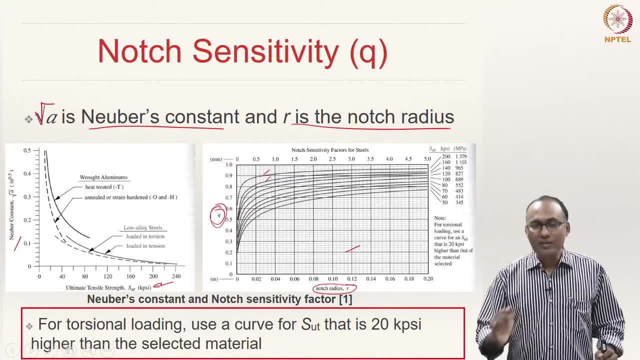 So you can calculate what is the Q for the given material and knowing the geometry, and then you will be able to calculate theoretical stress concentration factor from the type of loading and also the geometry. Once having these two parameters, then you can calculate your fatigue stress concentration factor: K f, that equal to 1 plus Q times K, T minus. 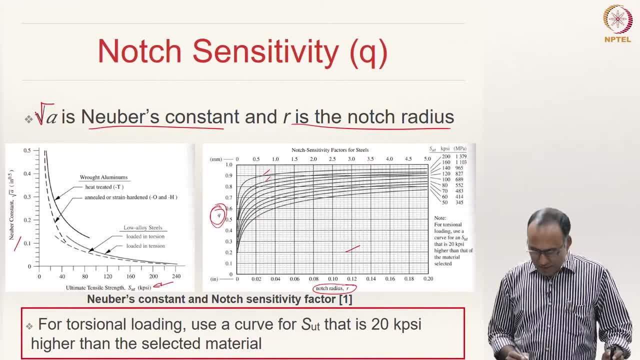 1, right. And if your loading is torsional loading, then what you need to you do is you need to. if the material's ultimate tensile strength is 100 k psi, you need to add 20 k psi to that and take that as your material to calculate Q. that is only to be done when. 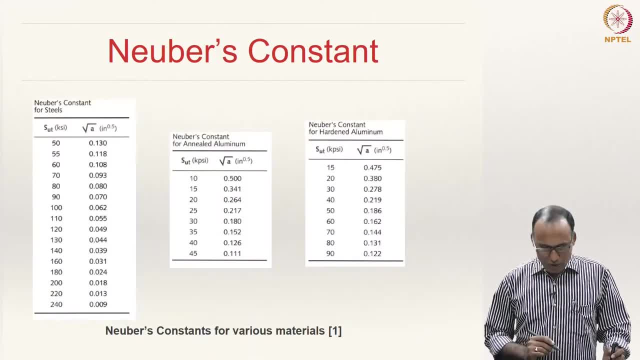 you are when you are doing torsional loading. Alright, So this is…. These are the tables that are available for Neuber's constant for different materials. This is for steel, This is for annealed aluminum, This is for hardened aluminum, And then you can directly look at the table And then find out what. that is, This is a unit size learning table. It is a 20 inch LCD, isn't it? It is yours. This is a unit size learning table, So it is 20 inch LCD, And that, of course, it is different. 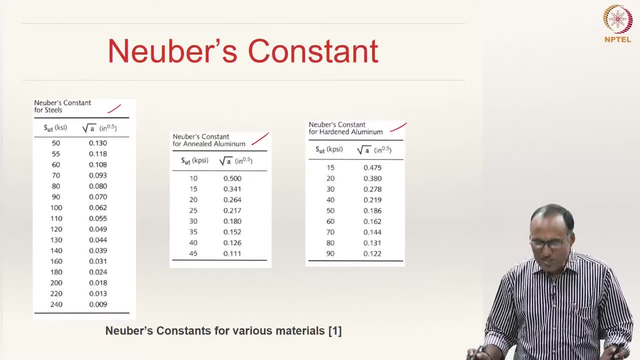 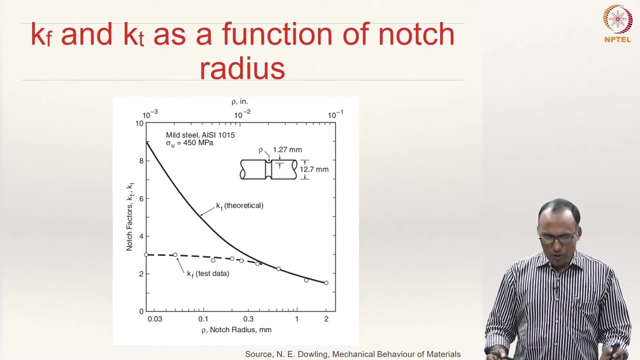 So Nalsost dramas include these two different tests. So this is for othersод find out the Neuberg's constant. and please note that Neuberg's constant is is not a, but square root a. So we can see that here we are looking at k f and k t as a function. 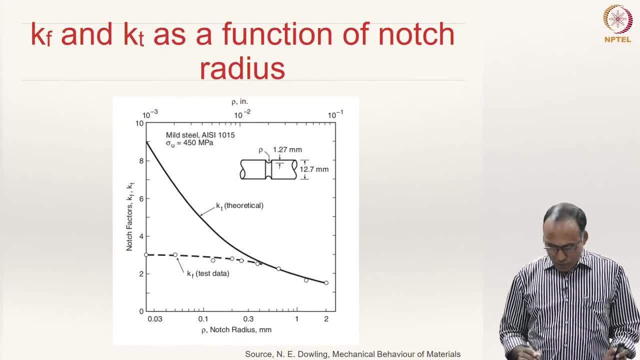 of notch radius As you reduce the notch radius. for larger values of notch radius, k f and k t are almost the same, but as you reduce the notch radius, then k, k, f becomes much smaller than k t And hence for smaller notch radius it is extremely important that you calculate. 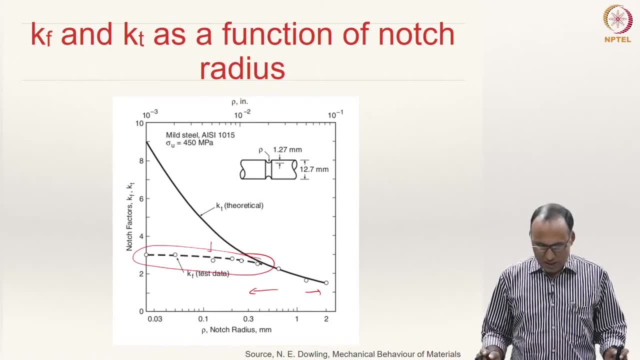 the value of k f. So, as we have already described, When rho becomes smaller and smaller- that means notch radius becomes smaller and smaller- then the materials notch sensitivity decreases, which means the locally the material is becoming more plastically deforming because of the lower notch radius and, as a result, it is becoming 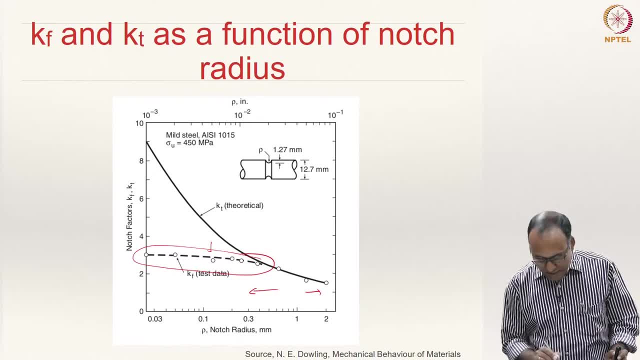 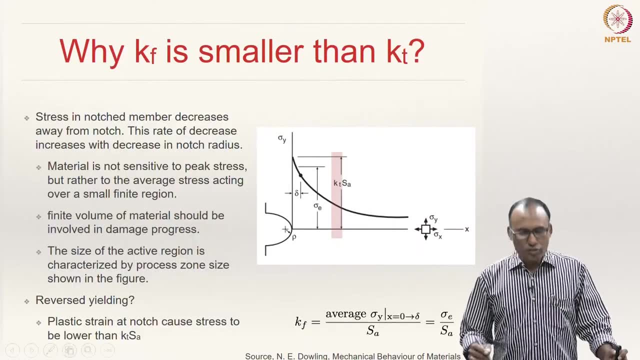 ductile and hence you need to account for this plastic deformation, and that is taken care of in the k f, whereas k t does not take that into account. alright, So now the question. So the question is: why is k f smaller than k t? as we have already discussed, 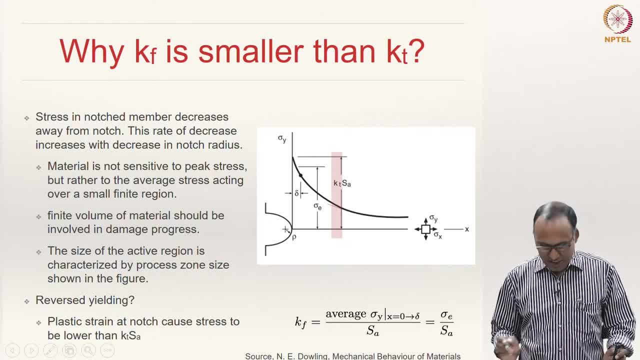 So stress in notch- remember- decreases away from the notch. as we can see clearly here. The rate of decrease increases with decrease in notch radius. as you reduce the notch radius, the rate of decrease increases. that means there will be a steep decrease of stress as you go away from the notch tip. 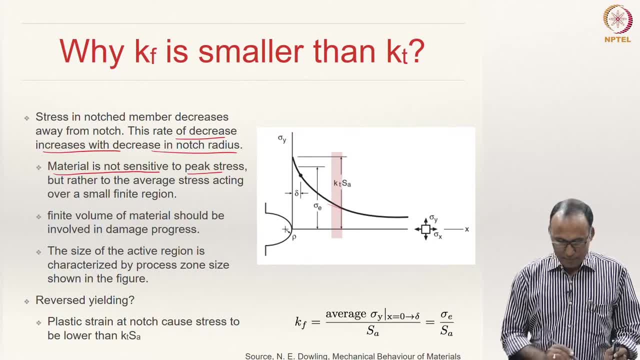 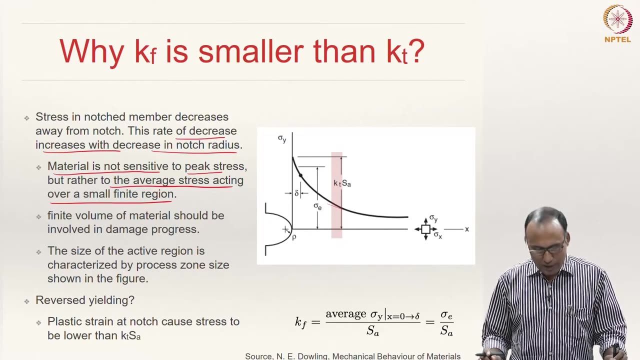 And the material is not sensitive to peak stress but rather to the average stress acting over a small, finite region. So you should not be. material failure under fatigue is not really dependent on the peak stress but on a average, small average volume ahead of the crack tip. 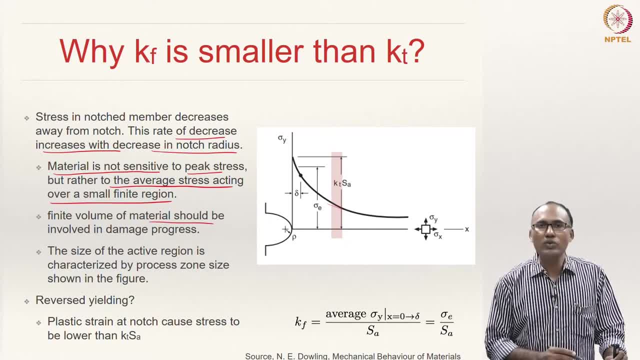 So the finite volume of the material should be considered which involve, which gets involved in the damage process. So the size of the active region is characterized by the process zone, as shown here, and then the plastic strain. So this particular stretch at a notch causes the stress to be lower than k, t, s, a. 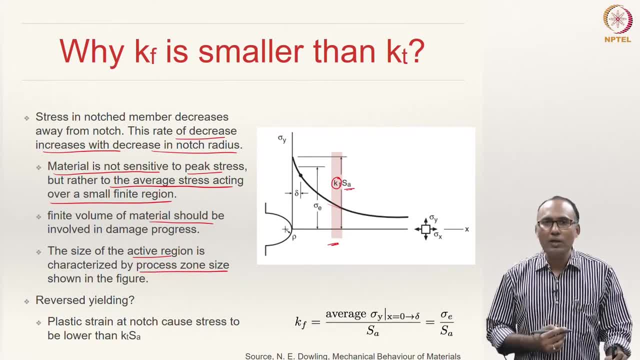 Normally, if your theoretical stress concentration factor is k t and stress amplitude is s a, then k t times s a is whatever actual stress amplitude experience by the material. but because of the plastic deformation this is not what is experience by the material- a little. 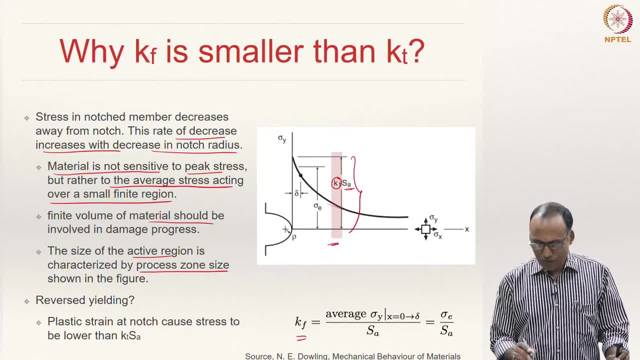 e less than that y when x is equal to 0 to delta. So x from 0 to delta. you have to take the average of this region and that turns out to be sigma e divided by S, e. that will give you your fatigue. 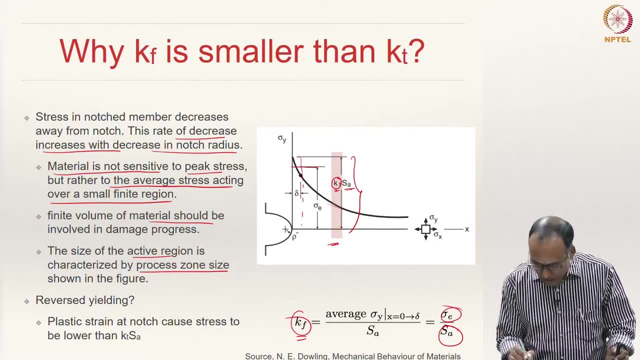 stress concentration factor And obviously that is going to be smaller than k t because you are only talking about this height in compared to that height. So it is coming primarily from not the maximum value but the fact that you need to consider the damage. 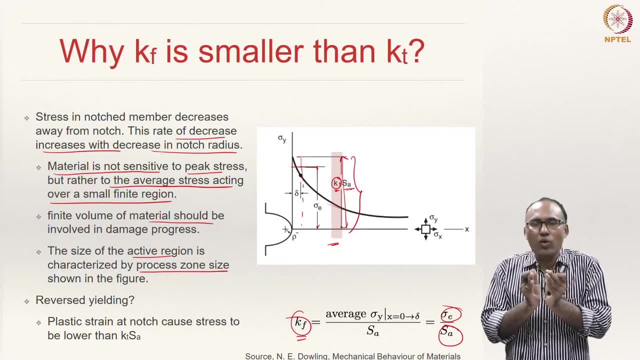 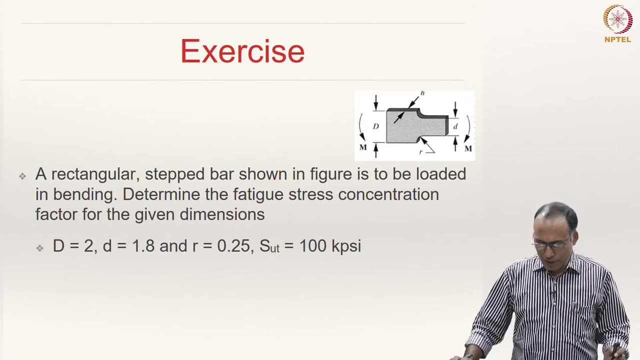 happens over a small region and you need to consider the small volume of the material in which the damage is taking place. As a result, you will have k f being less than the value of theoretical stress concentration factor. So this is an exercise problem that you are required to try solving on your own, wherein 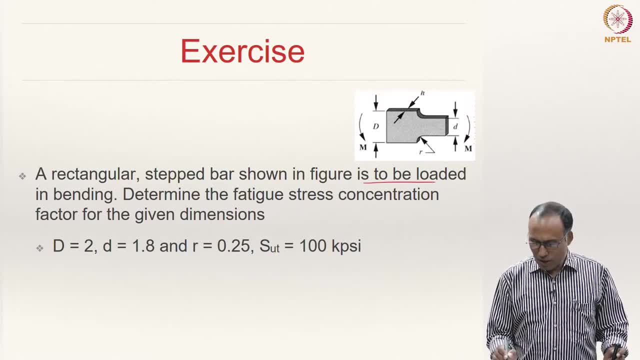 you have a rectangular stepped bar as shown in figure. It is to be loaded in bed, So the bending, the kind of loading is given. determine the fatigue stress concentration factor. In order to calculate fatigue stress concentration factor, k f equal to 1 plus. 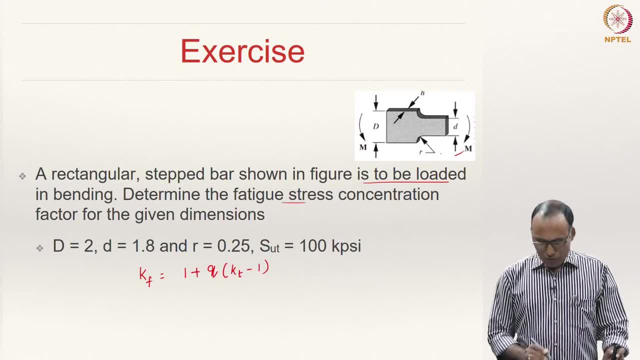 q times k t minus 1.. So now, first thing that we need to find out is: what is k t? How do we go about finding k t? You go back and so it is a rectangular cross section and bending, and capital D and small d are given, r is also given, All are in consistent units. 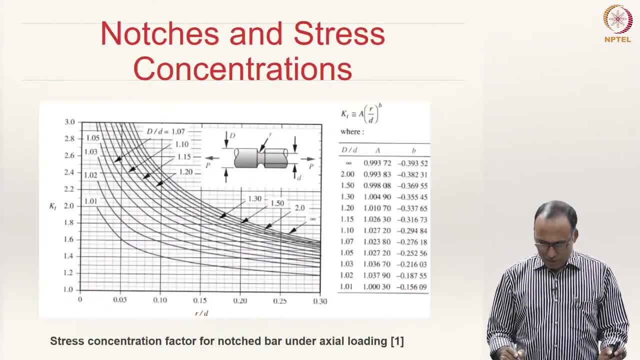 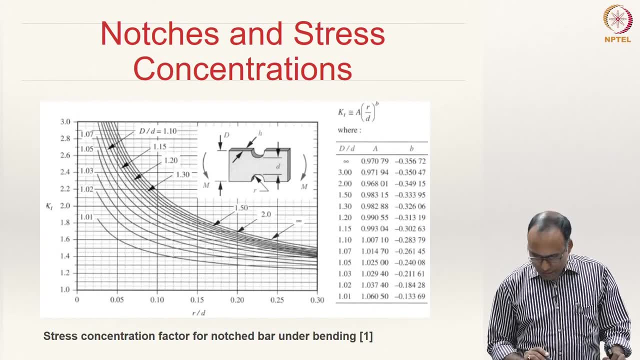 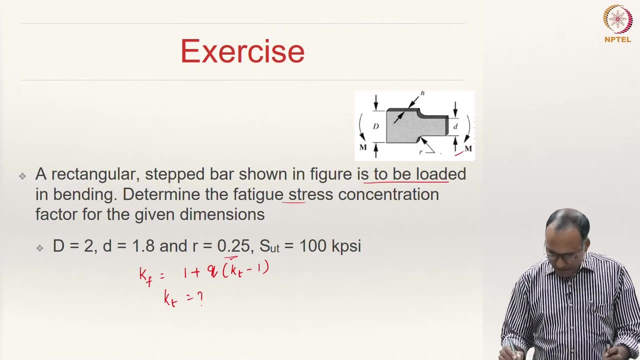 So let us go back and see one of the graphs. So here we have got r equal to capital D by small d. Capital D was how much? Let me check: Capital D is 2, small d is 1.8.. So 2 by 1.8.. 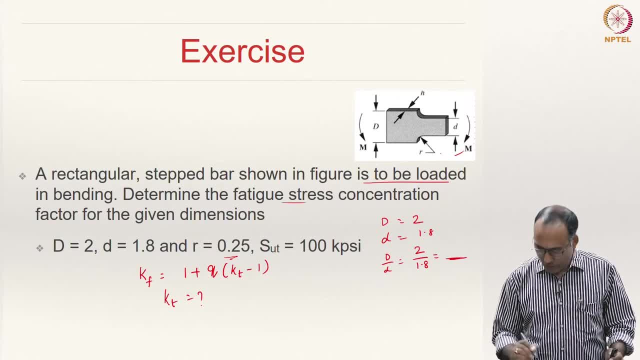 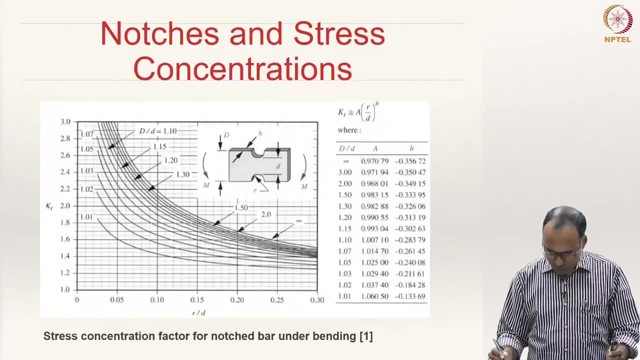 So that is what. for that, corresponding to that, you need to calculate. So that is one point, something right, And then so somewhere here, and then you know what is A and what is B. So after finding out these values, let us say it is 1.1 approximately. So you, 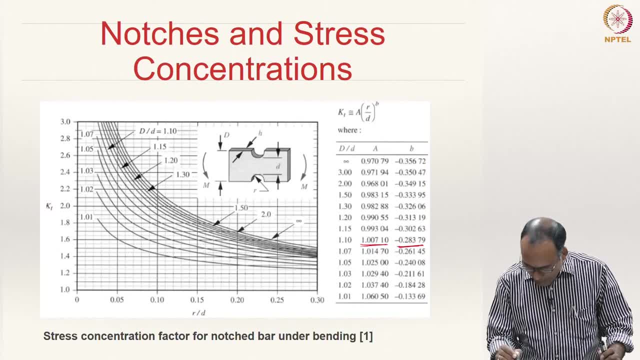 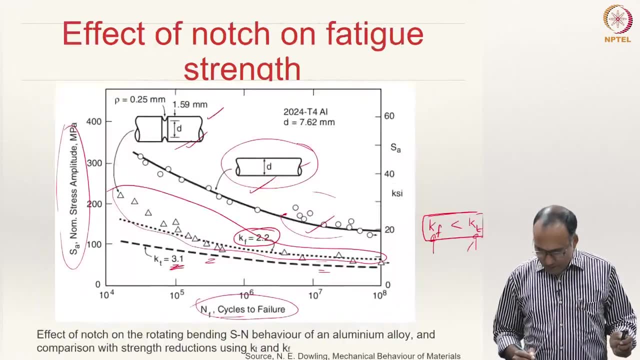 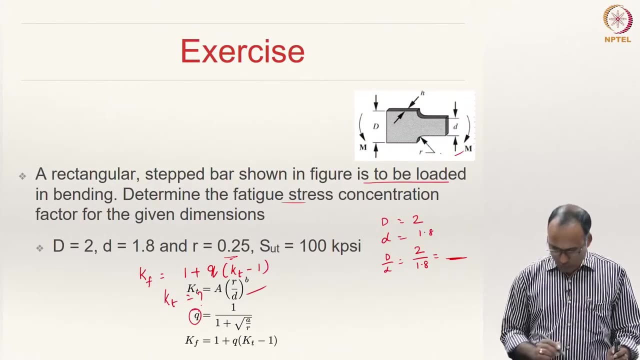 know what is A and what is B. Then after finding out those two values, then you will plug that in this equation: A and B are known. Now you know what is r and what is D in consistent units and then plug that in and you get your k, t And now we need to calculate q. q depends. 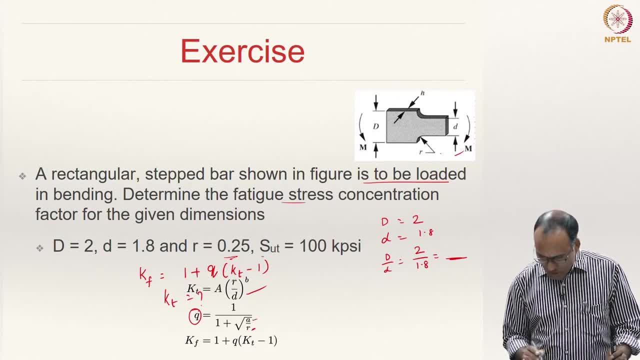 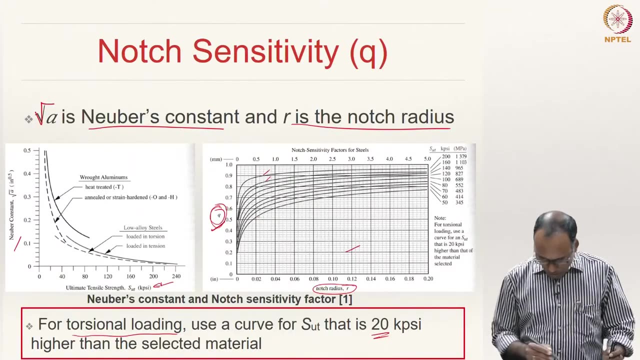 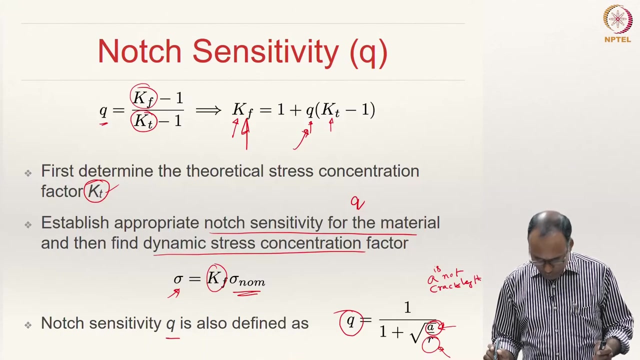 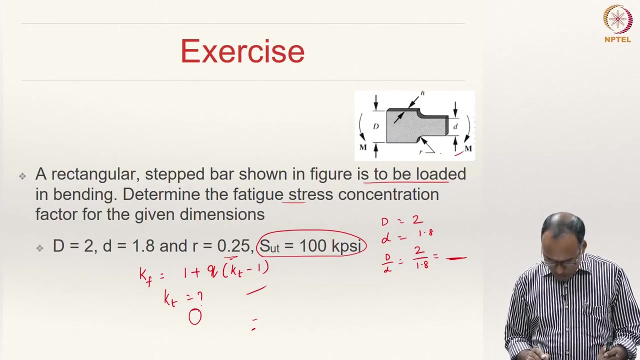 on A and r. r is known For s? u t equal to 100 k psi. we need to find out what is q. right, So you go back. So we know. the notch radius is equal to 0.25 inches. No, no, 0.25.. Okay, So now let us. 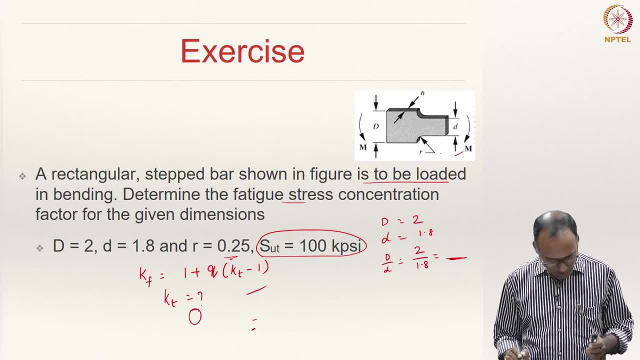 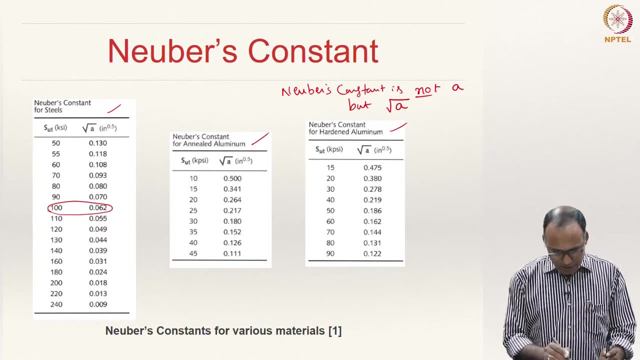 calculate. Let us calculate Neuber's constant for s? u t equal to 100 k psi. So for s? u t equal to 100 k psi, Neuber's radius is this and use that 0.062.. So 1 by 1 plus square root.